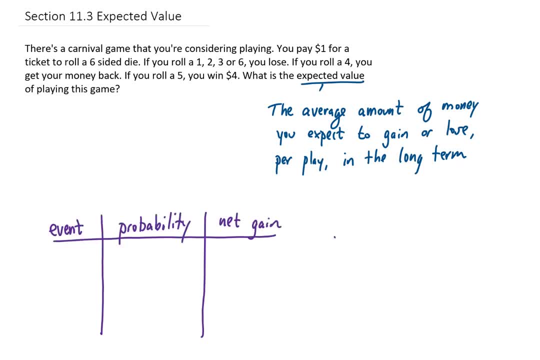 To answer this question, it might be best to make a chart And in this chart we're going to list the event that happens, the probability that that event happens and the net gain from that event happening. So we're rolling a die, so the possibilities are rolling a 1, a 2, a 3, a 4, a 5, and a 6.. 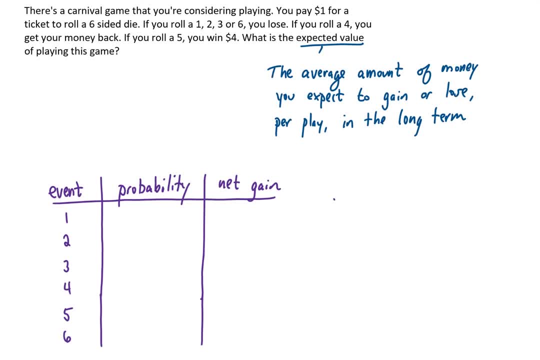 The probability of each one of those events happening, if this die is fair, is 1- sixth: There are six possible outcomes, so the probability of any individual outcome is just going to be 1 out of 6.. Now about the net gain With this game. if we roll a 1,, a 2,, a 3, or a 6,, we lose. 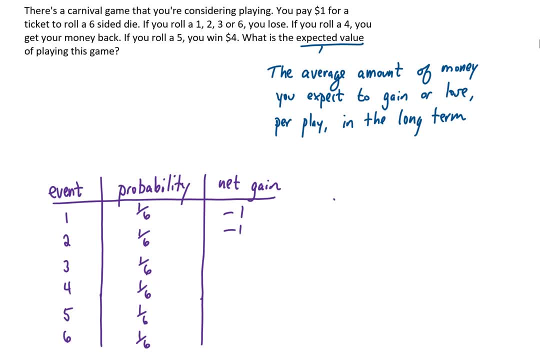 so we lose a dollar. So in the row for rolling a one, a two, a three and a six, I'm going to put a net gain of minus one dollar. If you roll a four, you'll notice you get your money back. so there's no gain or loss there. 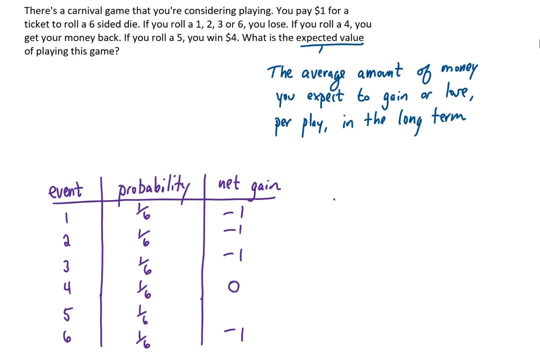 And if you roll a five, you win four dollars, but notice that you paid a dollar. so our net gain is actually just three dollars there. Now to calculate our expected value, we're going to take every probability in this table and multiply it by the net gain in that table. 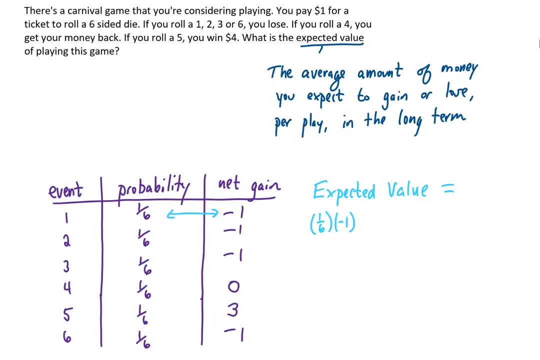 For example, for this first row rolling a one, we're going to take one sixth and multiply that by negative one. We're going to do this in every single row and we're going to add all of our results together and that number is going to be our expected value. 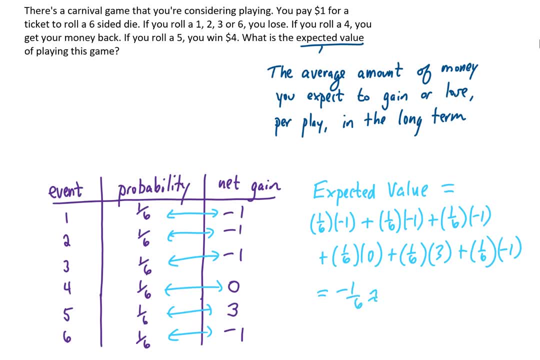 If we do this, we get negative one sixth, or we can get a decimal of negative .16667.. That is the expected value of playing this game. Now let's interpret it Well. what this means is that, on average, in the long run, we expect to lose. 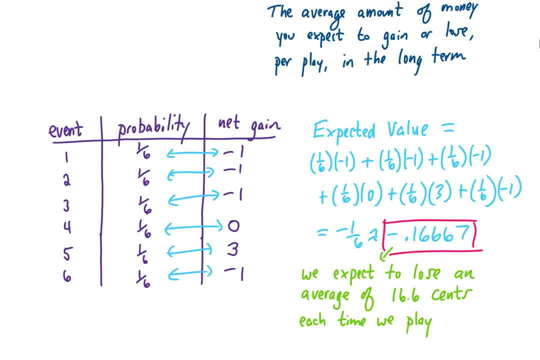 .16667.. That's $66 each time we play. That corresponds to 16.6 cents lost every time we play this game. Now, obviously, we will never lose exactly 16.6 cents in any given play of this game. 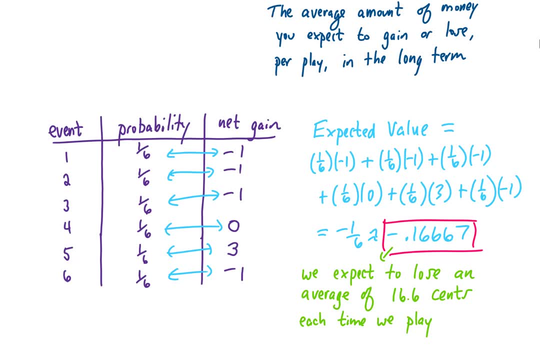 We can either lose a dollar or gain three dollars. But what this means is, if we play this game, say, a hundred times, we should expect to lose about $16 to $17 by playing this game. So we might say that this game is unfair because the people who play it are expected to lose. 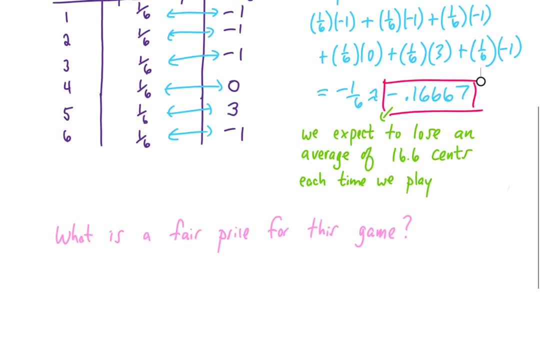 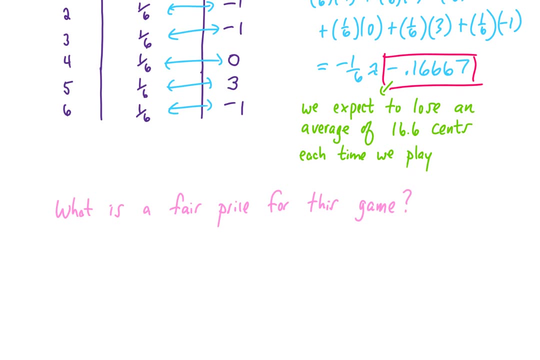 So a question we might ask is what would be a fair price for this game? Well, we paid $1 for our ticket and given that we're paying $1 for our ticket, our expected value is to lose 16.6 cents per play. 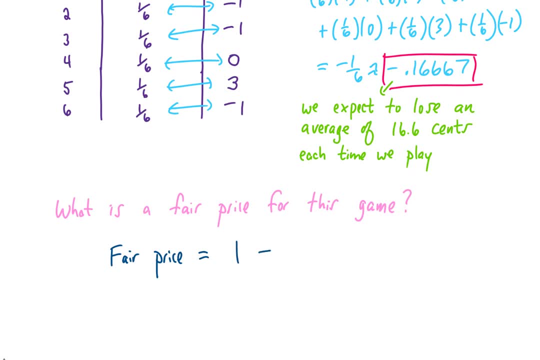 So it might make sense that if we take that $1 fee for playing this game and subtract off the 16 cents that we expect to lose, that we might get a fair price for this game, And that would be correct. The fair price for this game is .8333 dollars, or about 83 cents. 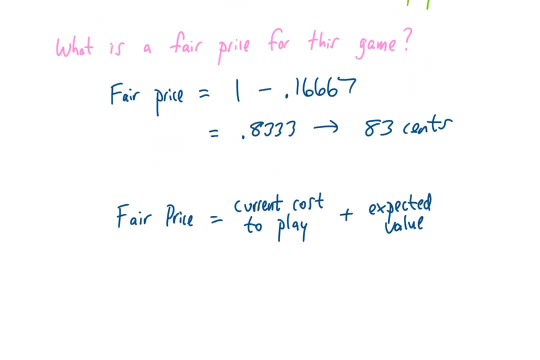 And, in general, the fair price for a game can be given by this formula: We just take the current cost to play the game, add on to that the expected value and you get yourself the fair price for playing that game. Okay, let's do a couple more examples. 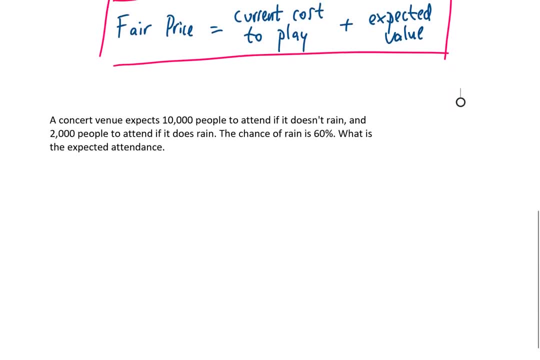 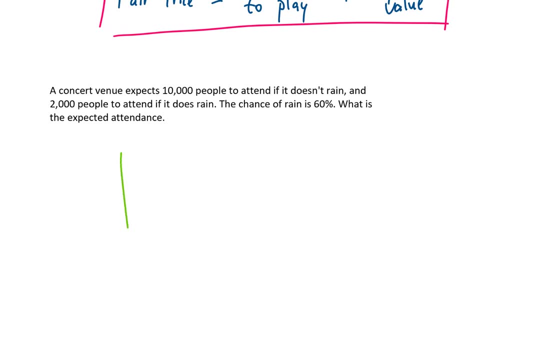 Here's an example: A concert venue expects 10,000 people to attend if it doesn't rain and 2,000 people to attend if it does rain. The chance of rain is 60%. What is the expected attendance? So we could make a table for this. There are two possible outcomes. 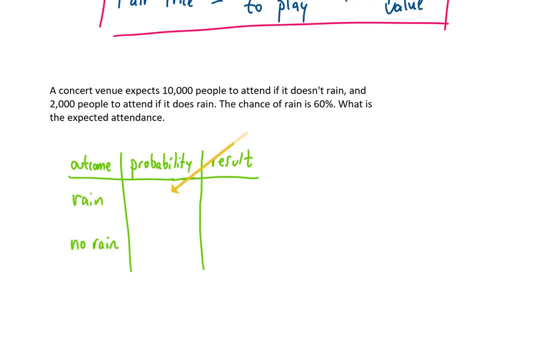 Either it rains or it doesn't. The probability of rain is said to be 60%, which we can write as .6. That means that the probability that it doesn't rain is 0.4 or 40%. The result if it rains is 2,000 people and the result if it doesn't rain is 10,000 people. 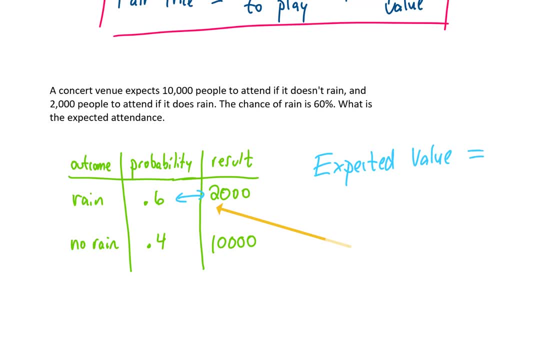 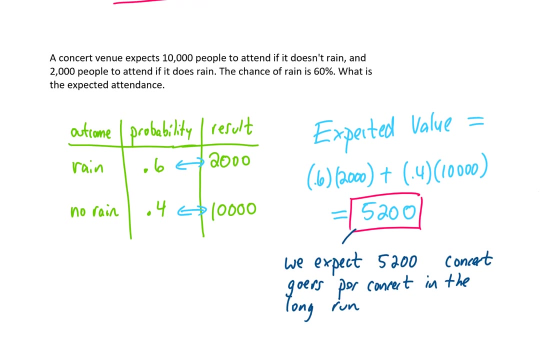 To calculate the expected value, we take each result and multiply it by its corresponding probability. We add those answers together, and when I do that, I get 5,200 attendees. Now, that is the answer. let's interpret it. What we just found was that, in the long run, under these conditions, we expect an average of 5,200 concertgoers per concert. 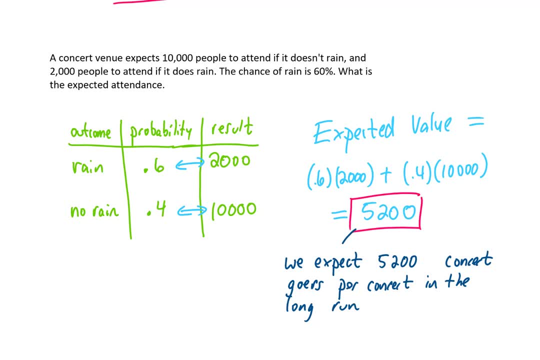 Now again. obviously you are never going to have exactly 5,200 concertgoers. We are assuming we are either going to get 10,000 or 2,000. But on average, given that there is a 60% chance of rain, we should expect 5,200 concertgoers in the long run. 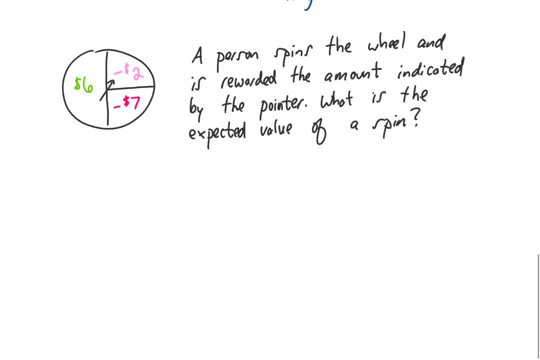 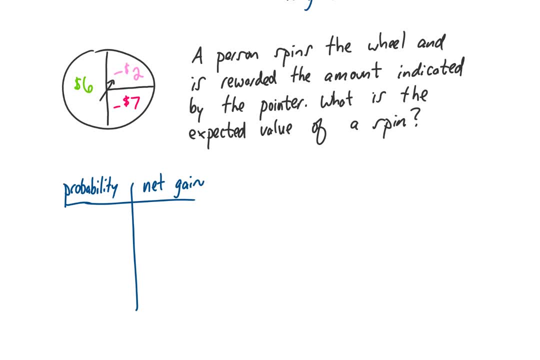 We need probability and we need how much we are winning or losing. So the idea from this drawing is that you should have a 50-50 chance to win 6 dollars, Because if this is a fair spinner, 50% of the spins will land on this 6 dollar, half of the pie.